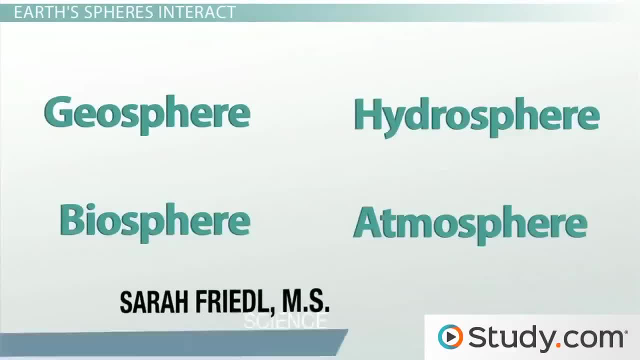 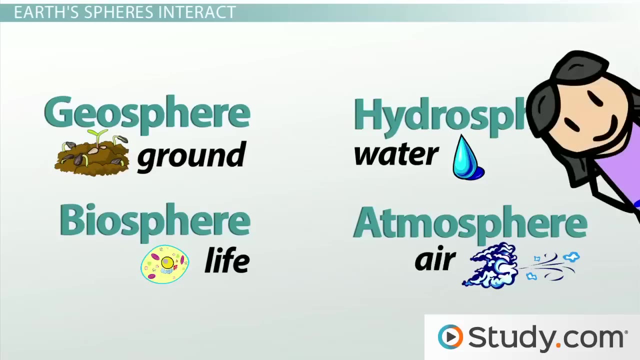 In another lesson we learned about Earth's four spheres. These are the geosphere, hydrosphere, biosphere and atmosphere. Together they make up all of the components of our planet, both living and nonliving, And while we can describe, 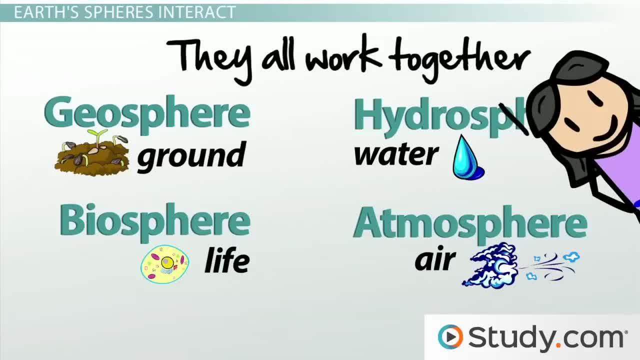 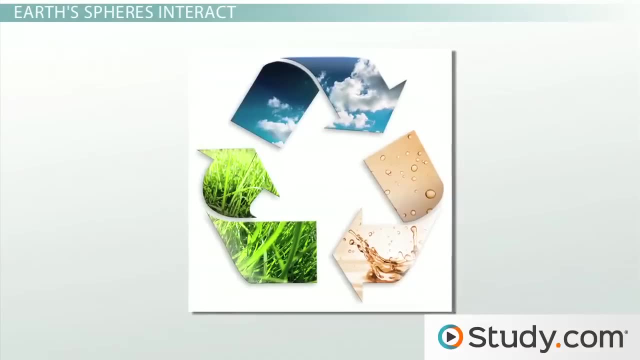 each individually in terms of its properties and features. you'd have a difficult time finding an example where one sphere doesn't either touch or interact with at least one other. This is important because these interactions are what drive Earth's processes. Material on Earth doesn't stay how it is: it gets. 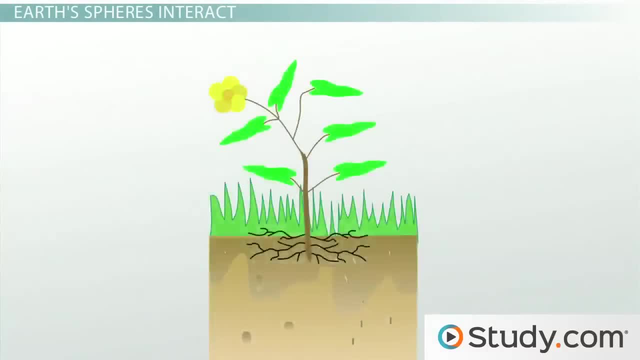 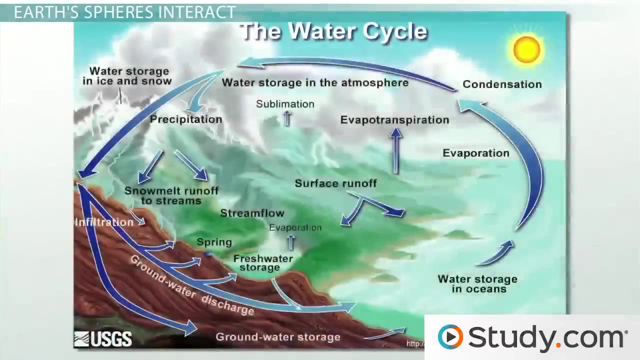 recycled into other phases and forms. Plants in the ground die and, as they're broken down by microorganisms, they become soil, which can then feed new plants. Water cycles through different phases and locations, like when it evaporates from the oceans and then rains down onto the ground or into a 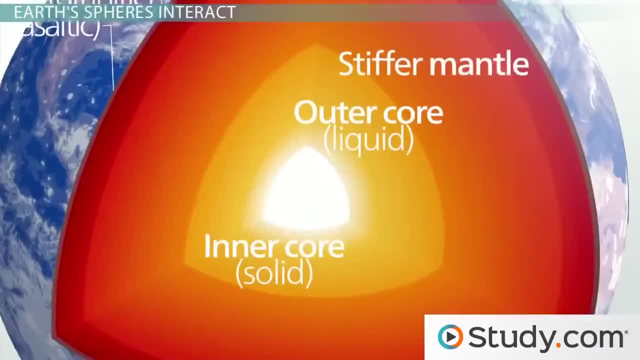 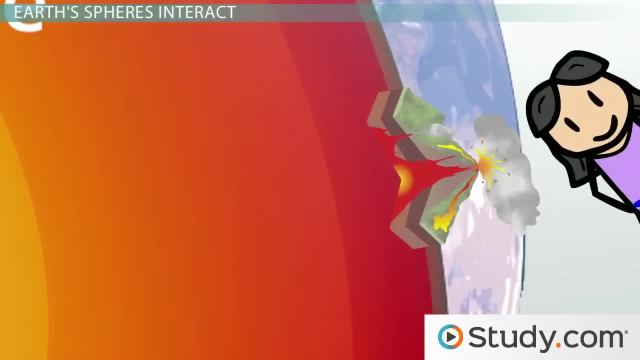 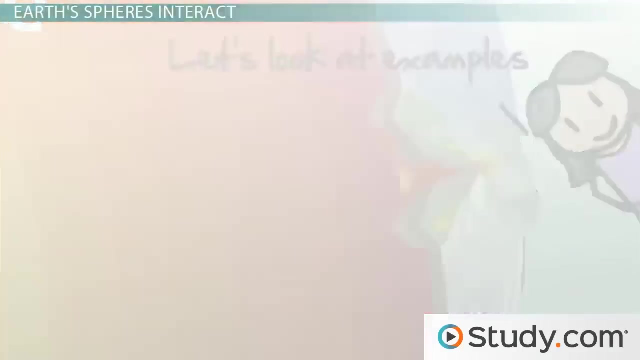 lake Rock also gets recycled under earth's surface, where it is melted down and then sent back up in volcanic eruptions. So now that you know why this is important, let's look at some examples of how these interactions occur between the four spheres of Earth. Pretty much any event on Earth is going to involve more than 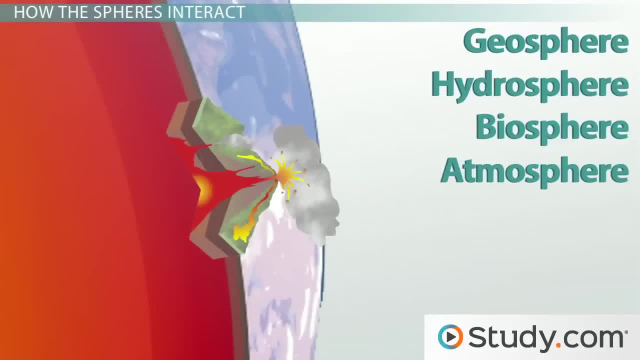 one sphere. Let's look at a fairly simple example to begin with, volcanoes. Volcano eruptions are events in the geosphere, because this is both rock being pushed out from underground很 from under the surface, as well as a change in the surface land itself. 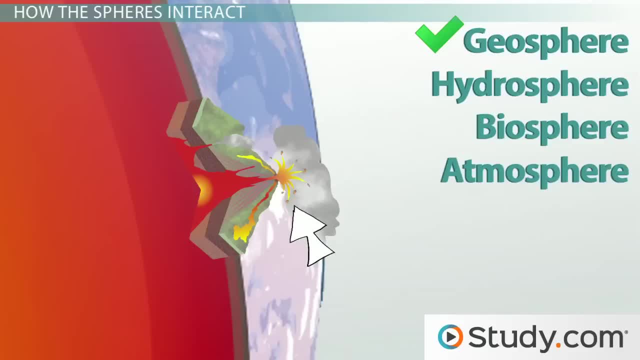 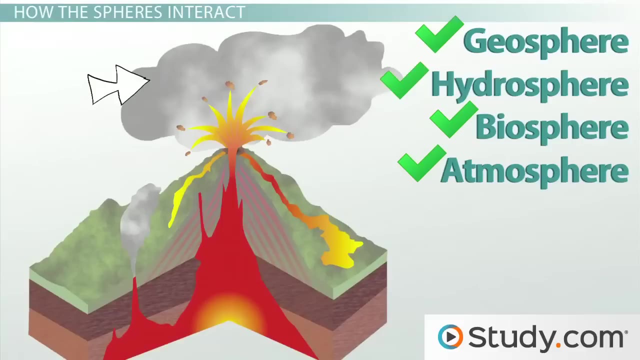 Volcanoes also spew a lot of gas and particulate matter into the atmosphere, as well as send hot lava flowing down mountainsides, disrupting the biosphere. Water will condense around that particulate matter in the atmosphere, so now we've involved the hydrosphere as well. You can see how this simple example. 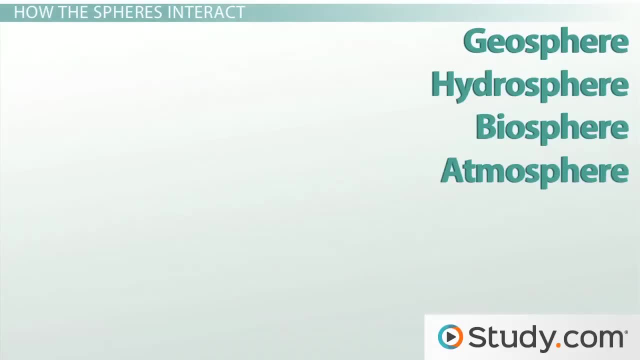 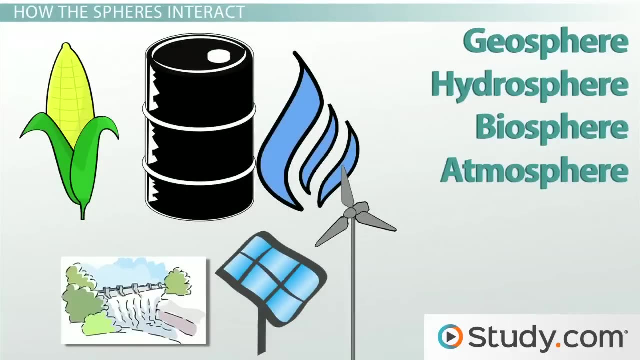 quickly got quite complicated. Let's look at another event to see how the spheres interact. Humans use a variety of natural resources to generate power, such as plant material, oil, natural gas, wind, water and sunlight. You can see right away that we've involved all of the spheres already, even before we started talking. 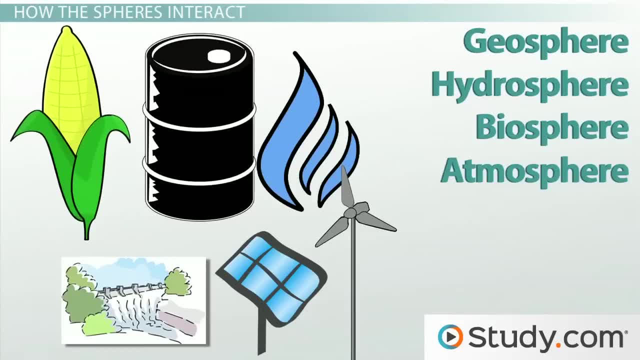 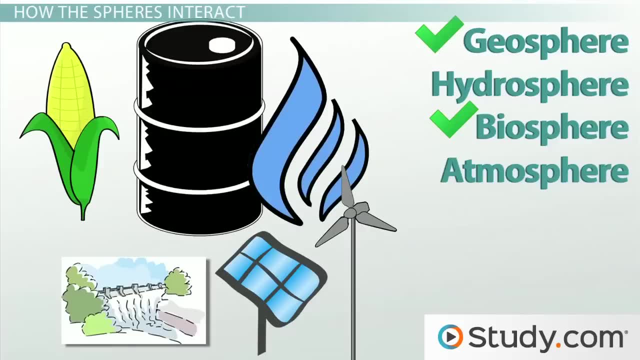 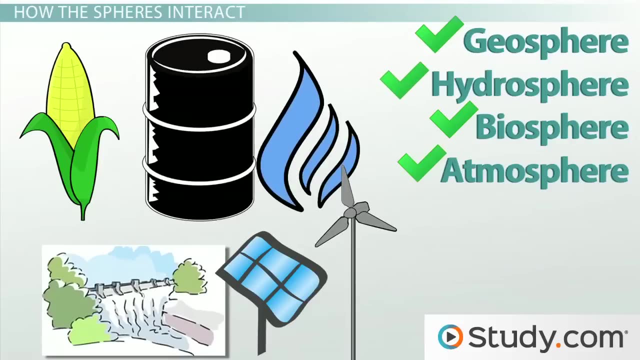 about how we harness these resources. We use corn for ethanol. the biosphere, oil and natural gas for heating homes and fueling cars, the geosphere and the wind, the atmosphere and water, the hydrosphere. Now let's look at an example. that's a bit trickier. 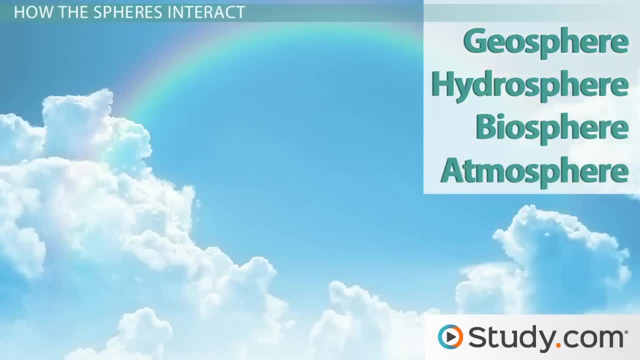 clouds. Clouds form when water droplets condense around dust particles in the air. But wait, does this mean that clouds are part of the hydrosphere because they're water, or does it mean that they belong to the atmosphere because they're? 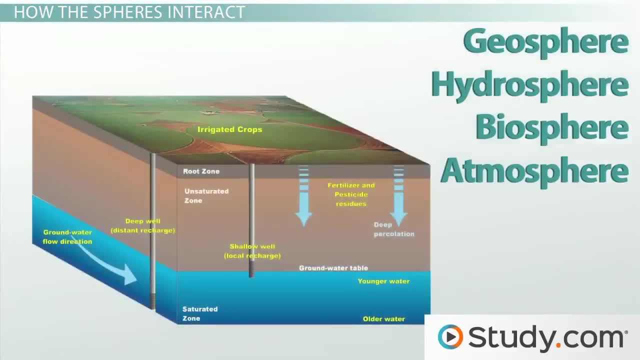 in the air. And what about ground water? Is this part of the geosphere because it's in the ground, or considered part of the hydrosphere because it's still water, no matter where it's found? Or is it a source of hot water or just a liquid from digital geWORKS plants? 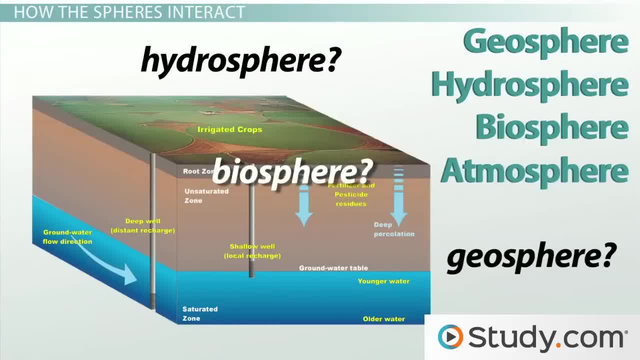 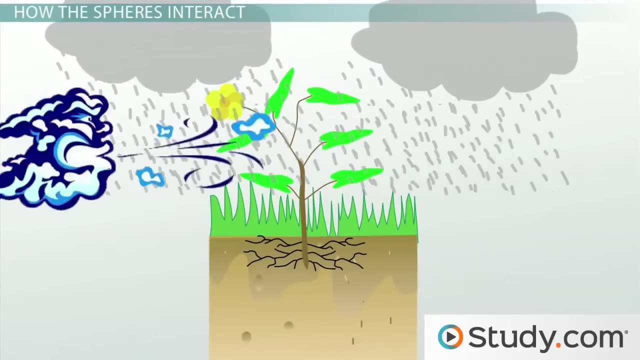 this part of the biosphere, because the soil is also filled with living things of all shapes and sizes. The biosphere is a major contributor to the recycling of other material and earth through different spheres. Take plants, for example. they drink liquid water from the ground and breathe it back into the 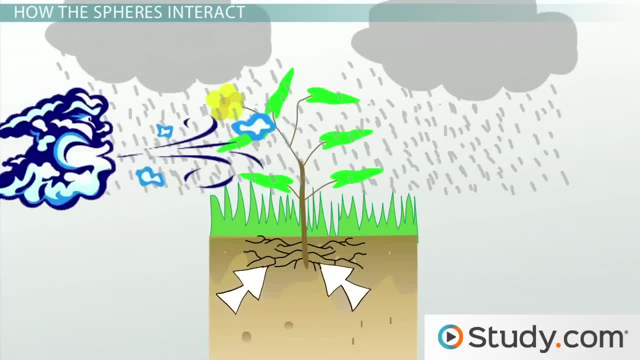 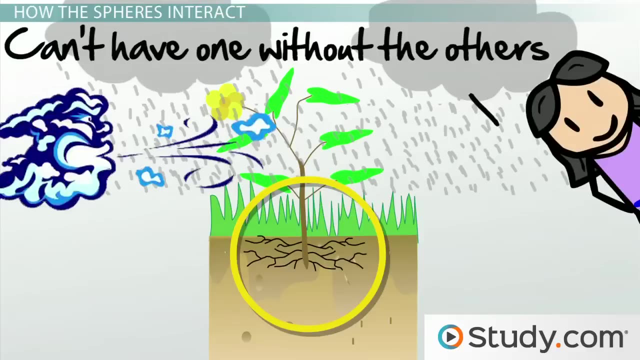 atmosphere as a gas. They also eat minerals from the soil and turn them into biological material, And in the geosphere, their roots help keep the ground in place, protecting it from wind and rain. As you can see, it's really difficult to tease apart where one sphere ends and another begins: Oceans. 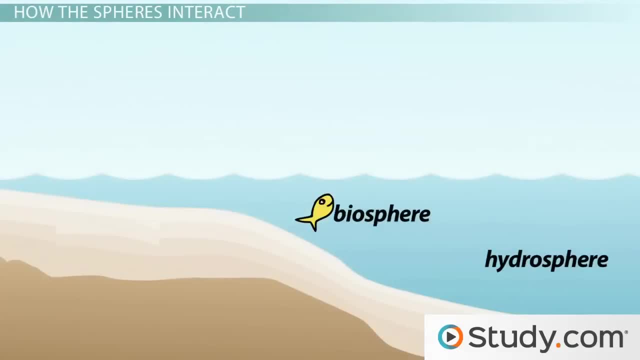 are filled with water, the hydrosphere and living organisms, the biosphere, but they also touch the sky, the atmosphere and the ground deep below the geosphere. Can you see how this makes each sphere important not only to each other, but to 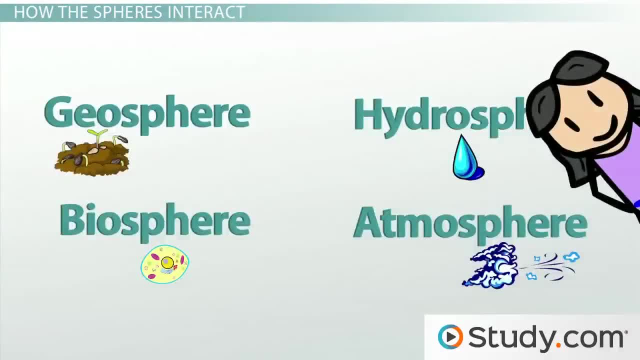 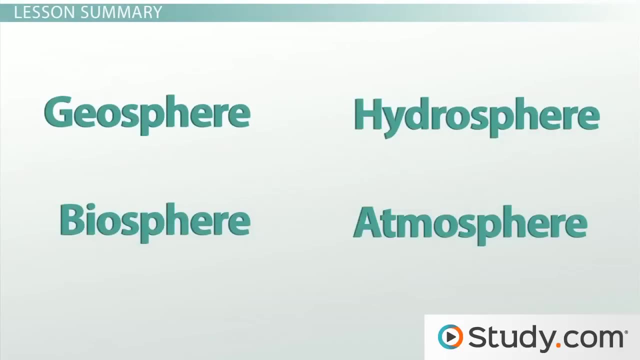 Earth as a whole. Earth depends on these interactions, And the balances among these interactions are what allow life to exist on our unique planet. Earth has four spheres called the geosphere, hydrosphere, biosphere and atmosphere. These spheres each have unique properties and features, but they 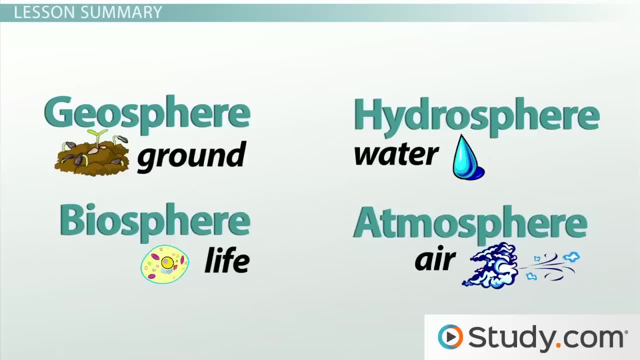 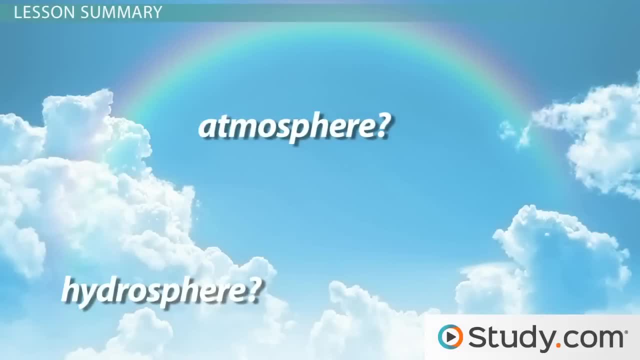 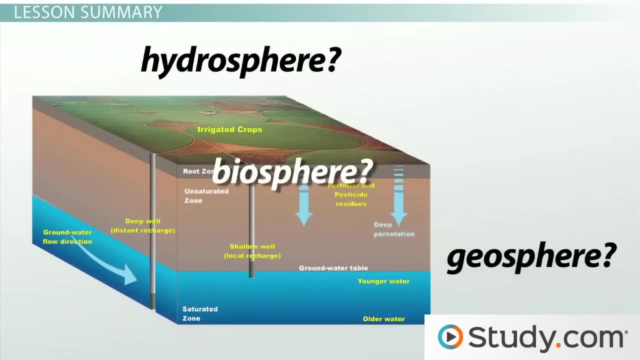 are not isolated on Earth, and they work together to drive the processes of the planet. Not only do each of the spheres constantly interact with the others, but it can often be difficult to tell exactly where one sphere ends and the other ends. Sometimes, multiple spheres can even occupy the same space, such as with clouds in the